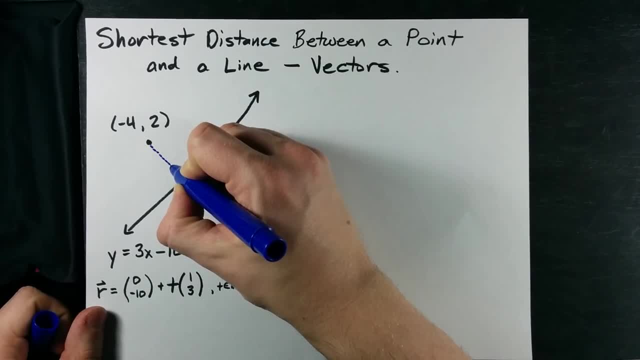 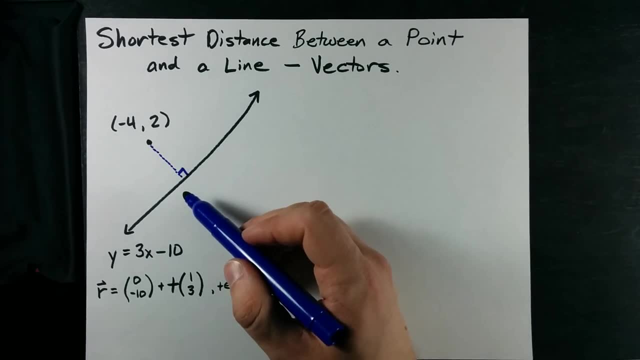 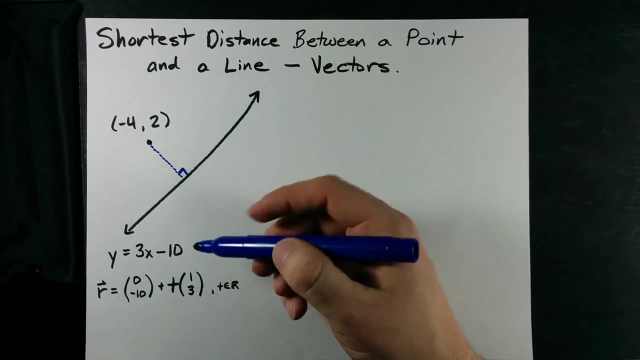 to this question is knowing that that shortest distance is this line segment which meets the line at a perpendicular or 90 degree angle. If you're feeling vector-y, the word might be orthogonal. Anyways, because I was given this equation of the line, I converted it to a vector equation. 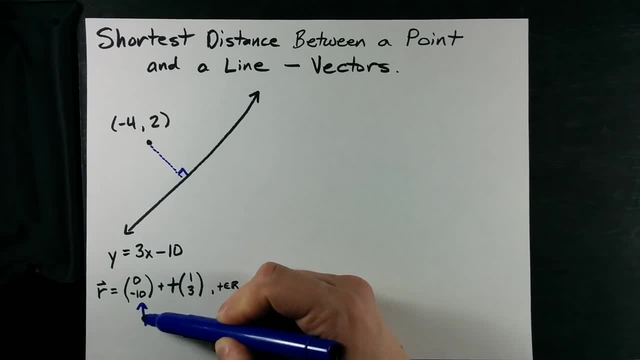 Here I have my position vector, which I've based on the y-intercept of 0, negative 10, and I've turned my slope into a direction vector. This slope up through the line is a direction vector. This slope up through the line is a direction vector. 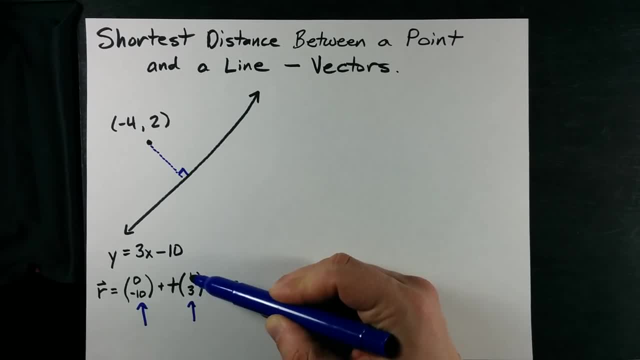 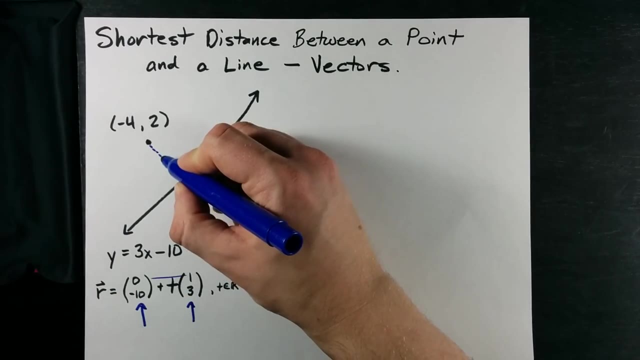 3 over 1 means I'm changing my y by 3 every time I change my x by 1.. This is my vector equation of the line. This is my parameter t. Anyways, where I'm going with that is that this line segment also has a vector equation. 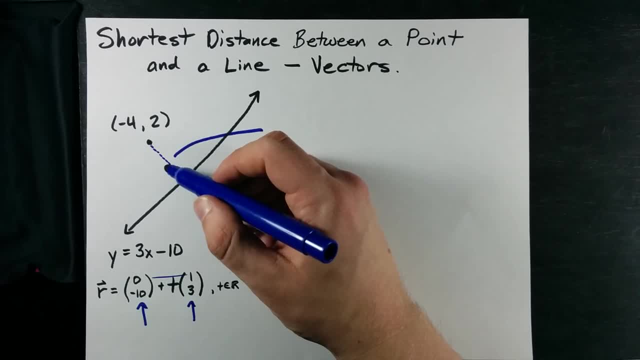 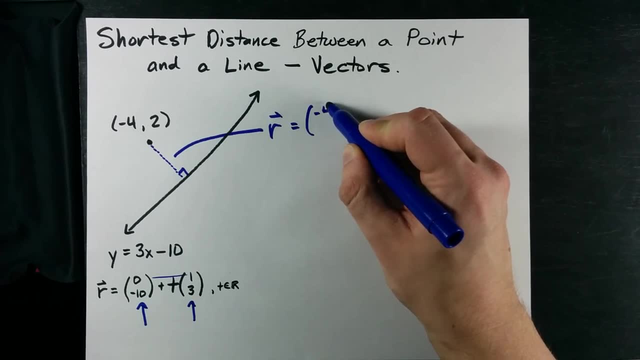 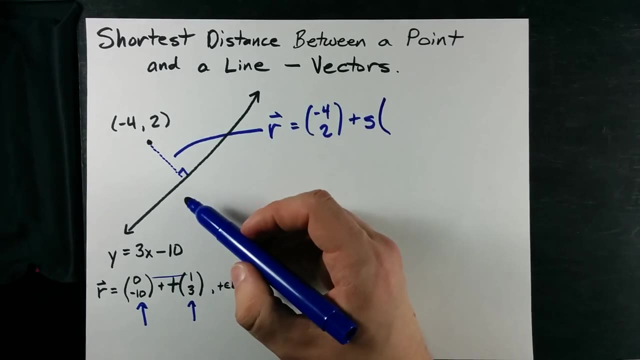 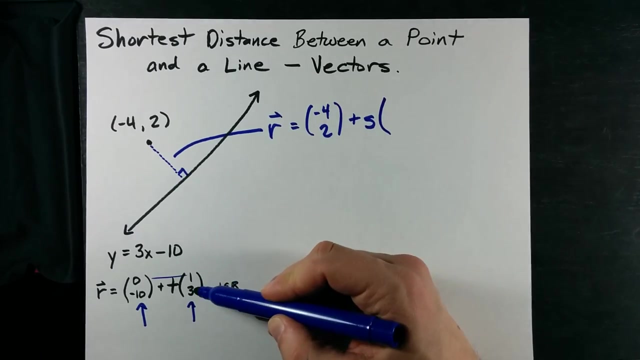 And what's awesome about this vector equation is that we've already been given a position vector That's negative, 4 comma 2.. I'm going to give it a different parameter s, And the direction vector for this needs to be orthogonal to this direction vector. 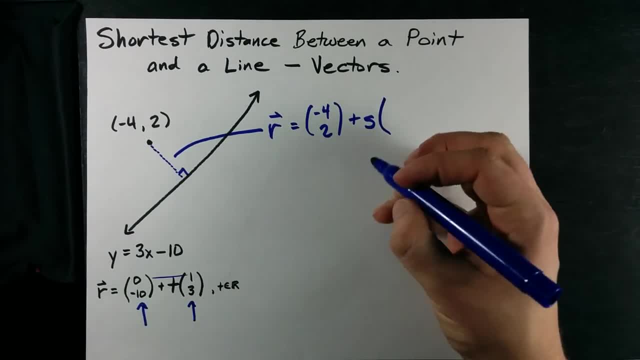 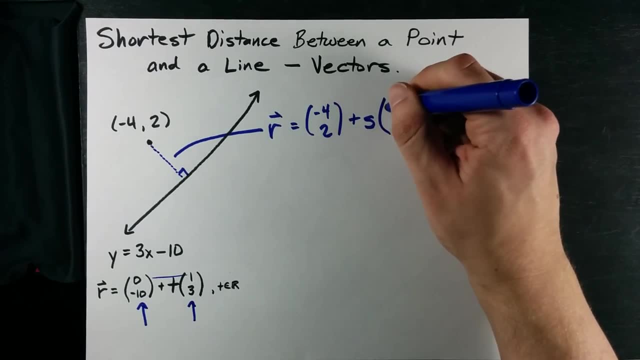 What that means is you flip the x and the y, so it becomes 3, 1, and you flip the sign on either of them. It doesn't matter which one I'm going to flip it. I'm going to flip it on this one, but it doesn't really matter. 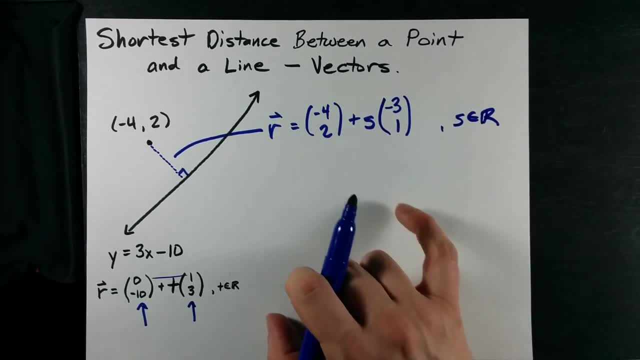 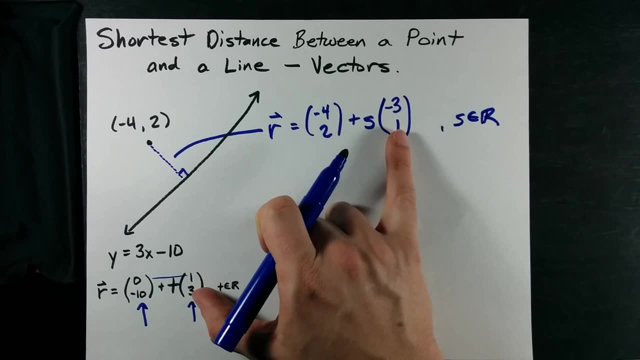 S can be any real number. The real key is that this dotted with this or the dot product of these two vectors needs to be 0. When the dot product is 0, they meet at a 90 degree angle, and that's the key. 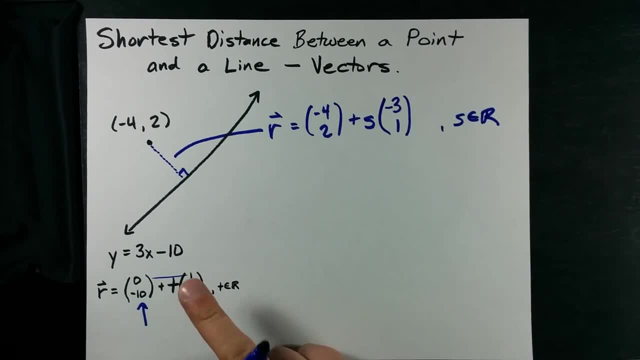 Pick any direction vector that dots with this to make a 0, and you're going to be fine. Now we already have the vector equations for the two lines. We simply need to do this. We need to find the point of intersection for both, like where the two lines intersect. 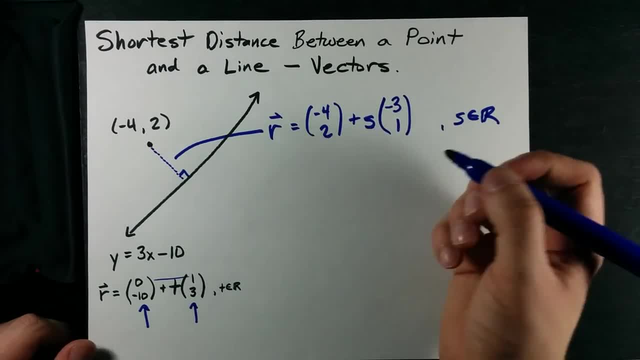 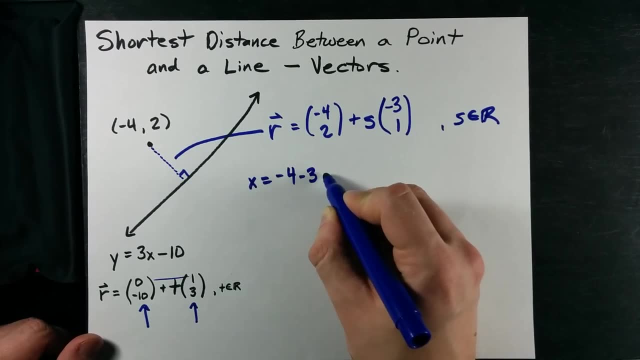 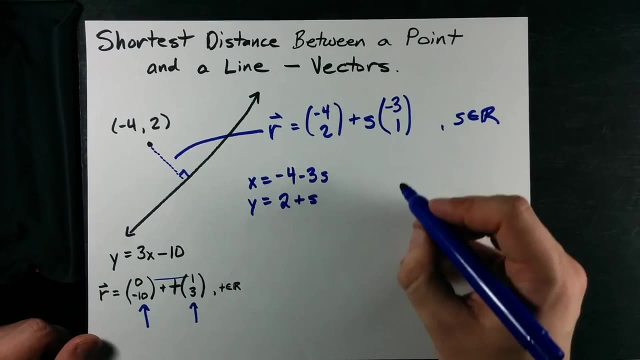 I'm going to do that with parametric equations because I feel like it and I'm in charge. My x for this equation is negative, 4 minus 3s, My y is 2 plus 1s And my other equation here is 0 plus t. 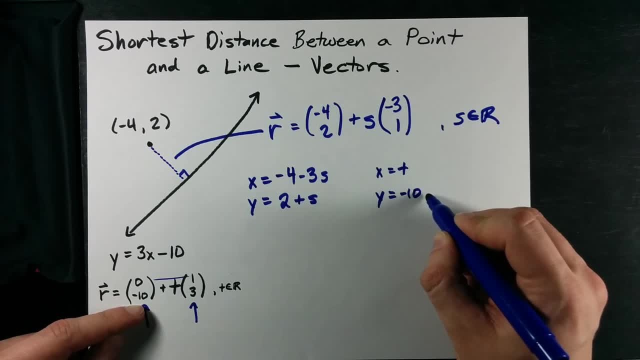 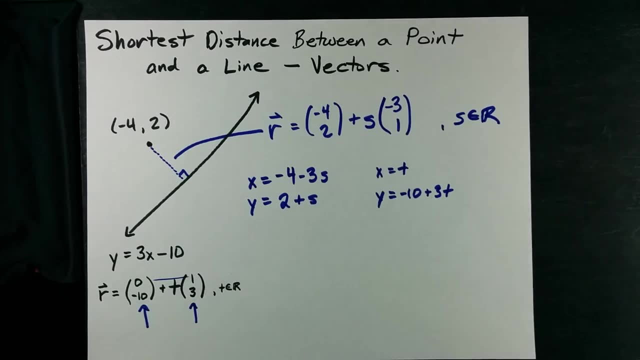 And my y is 2 plus 1s And my y is negative, 10 plus 3t. So how do I solve parametric equations? Let me see, if I remember this. I'm going to set my x's equal to each other. 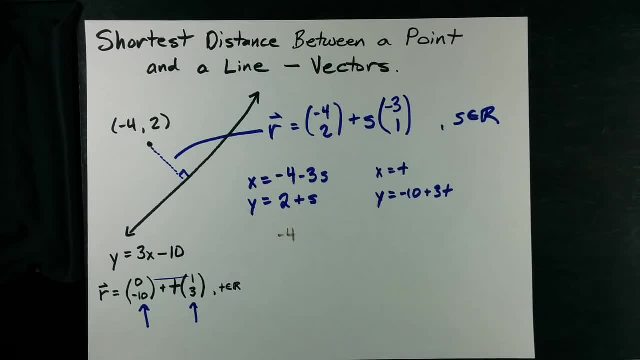 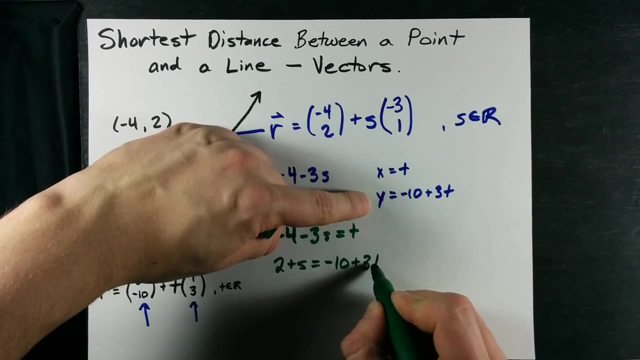 Wow, that marker is dead. Let's use green. Negative: 4 minus 3s equals t- Oh, that was easy. And 2 plus s- that's y- equals negative. 10 plus 3t- t is negative 4 minus 3s. 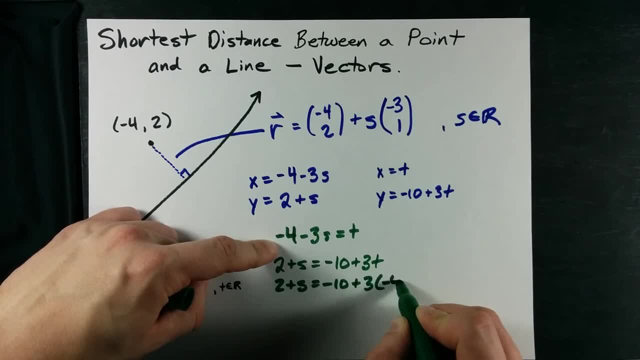 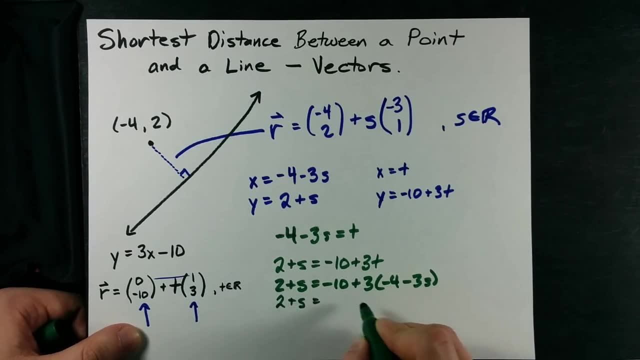 So I'm going to do a little substitution: Negative 4 minus 3s, wherever I saw t, And from here I believe it's just solving a linear equation. Negative 10 minus 12 minus 9s. That's me multiplying the 3 through. 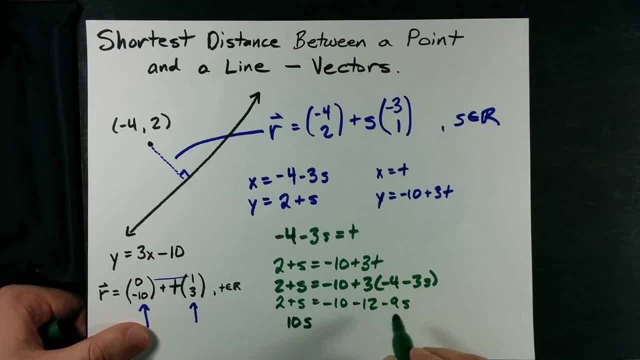 I'm going to put all my s's on one side, That's 10s. on the left, I'm going to put all my numbers on the other side: It's negative 24.. Yep, So my s turns out to be negative 2.4.. 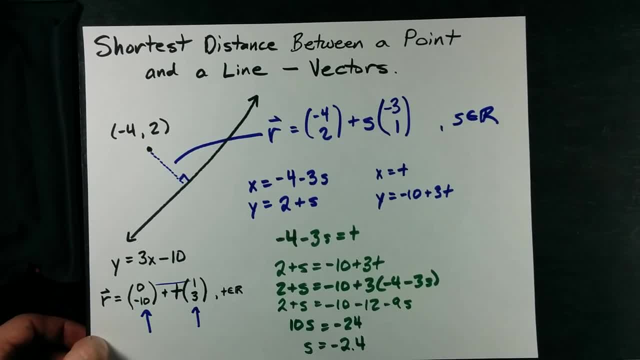 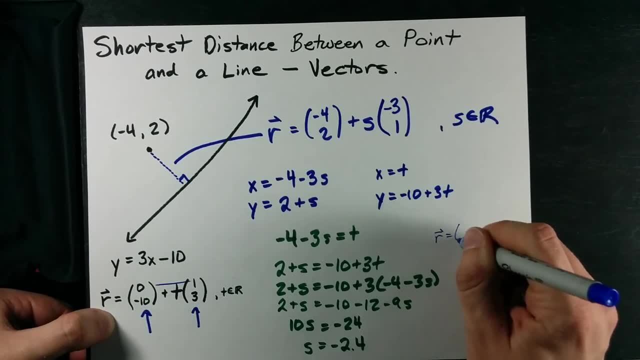 Sweet, I got one parameter. What that means is I just need to plug that s in to get the coordinates of the point of intersection. It's negative 4, 2, minus 2.4, negative 3, 1s. See how I.